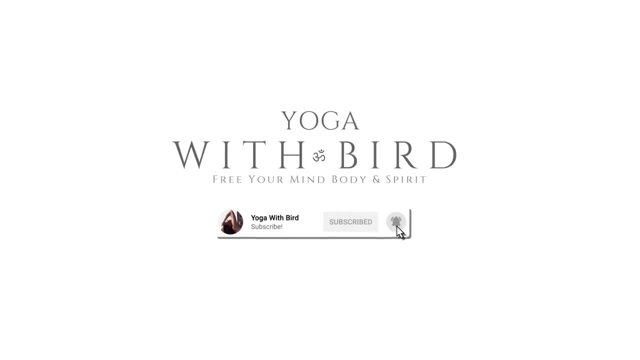 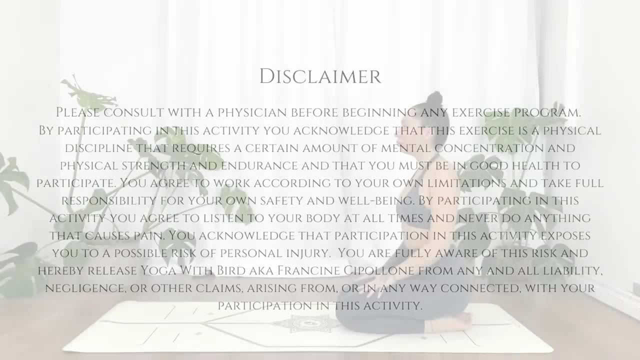 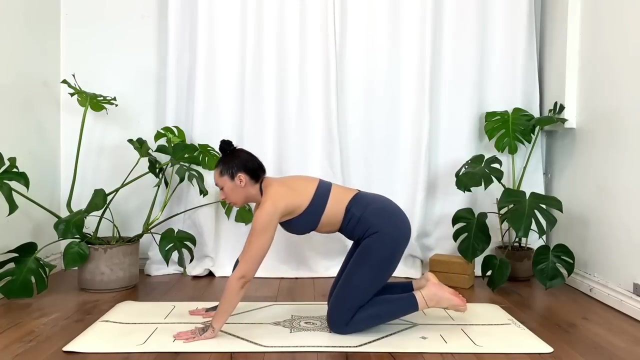 Welcome. As the title says, this is a 10-minute yoga to help you pass gas and go to the bathroom. Feel free at any point to skip any poses that don't feel right or modify if and when needed. We'll begin in a tabletop pose: wrists under shoulders, knees under hips. 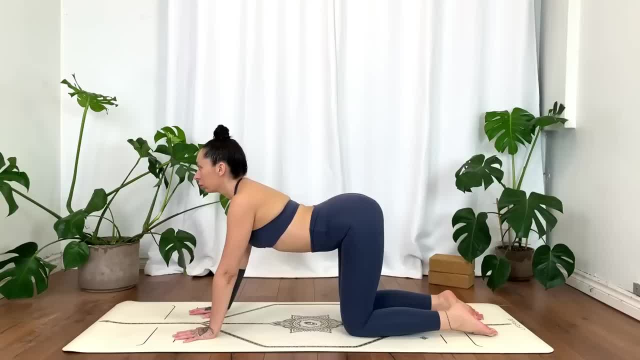 Dropping the belly. take your gaze up, inhale, Exhale, rounding through the spine. take your gaze down. We'll continue sinking breath with movement flowing at your own pace. We'll begin to find some organic movement, maybe circling the waist, rocking forward and back. 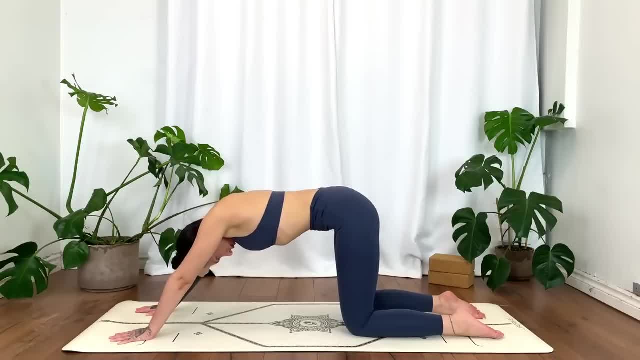 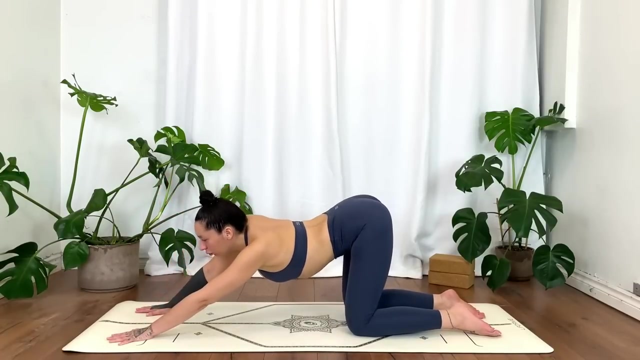 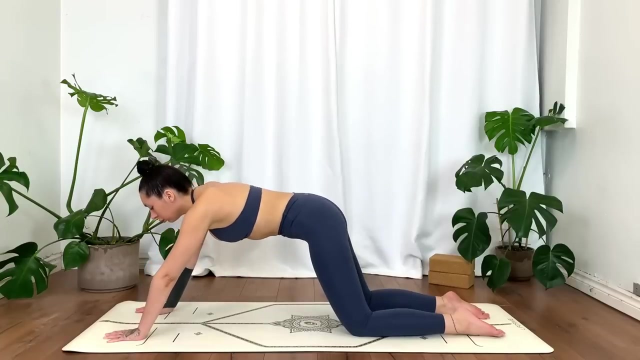 side to side. you can even walk the hands further forward towards the top of the mat. so just moving wherever the body needs to go here and wherever you are, we'll find a neutral spine. walk the hands as far up towards the top of the mat as you comfortably can as you start to melt the forehead down towards the mat for puppy pose. 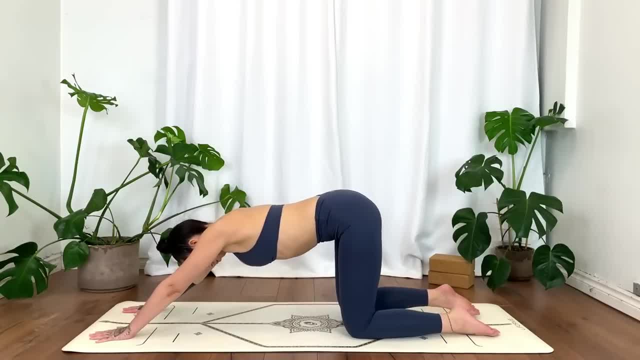 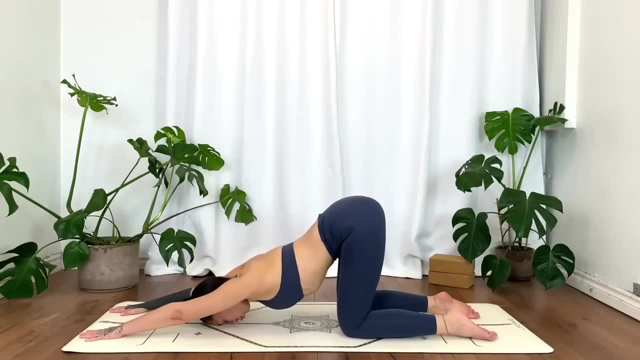 if you need a little more support or height. if this is too intense, you can place a block underneath the forehead, engaging, drawing the ribs in, but maybe softening the belly here, no clenching, of course. you can do that if you want to, pressing the tops of the feet into the mat, really engaging with the arms. 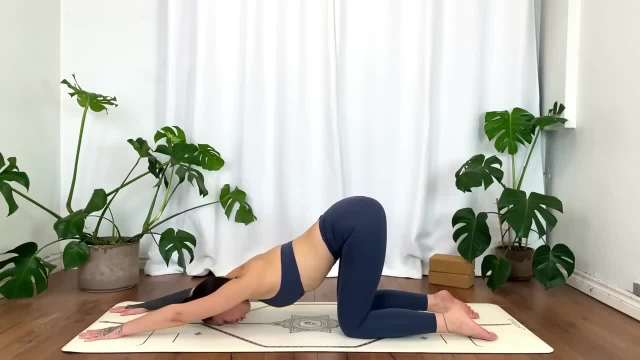 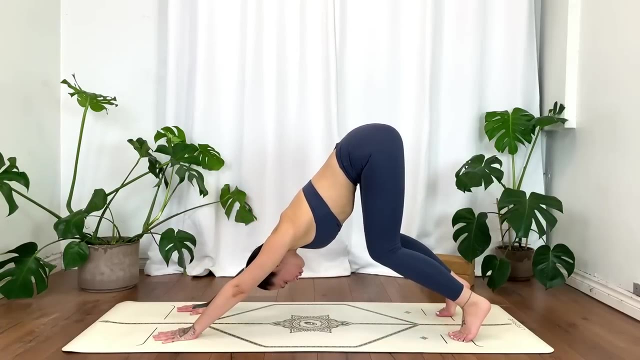 and we'll gently release. take your time. we'll tuck the toes, plant the hands under the shoulders as you send the hips up for down. dog, you can bend one knee, bend the other, just walk it out here, maybe rocking the hips. you can bend one knee, bend the other, just walk it out here, maybe rocking the hips up. 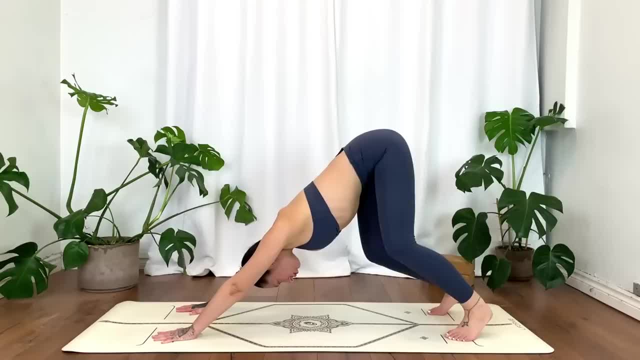 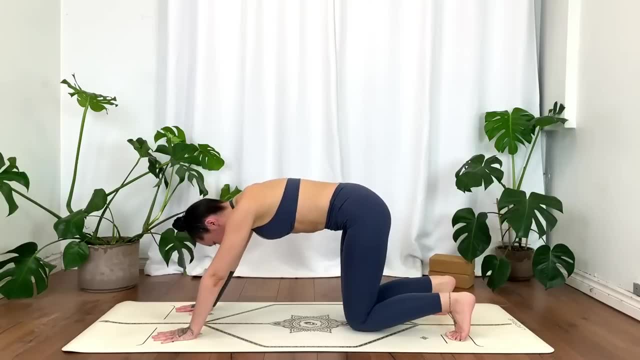 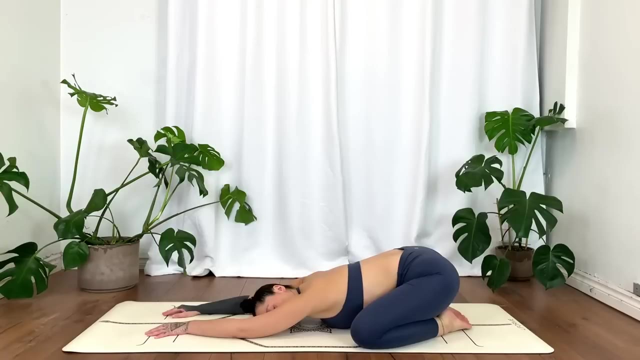 to side, bending the knees as much as you need, and we'll go ahead and plant the knees. coming into our child's pose, you can keep the knees closer together or take a wide leg child's pose, taking the forehead or cheek to the mat. option here to place pillows underneath the torso, underneath the hips, for added height and 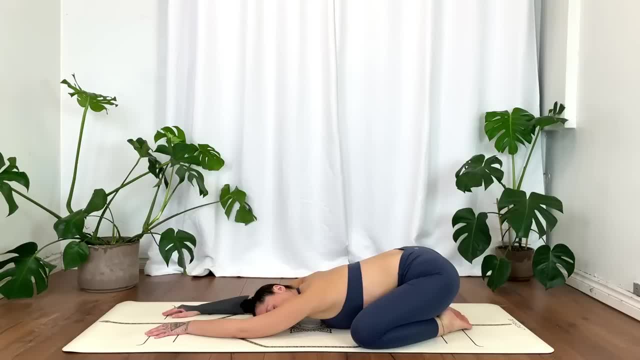 support. once again working with the breath to soften the body again- no clenching here- just being softening the belly, softening the lower back, the glutes, the hips, the ankles and the feet, softening the upper body, the shoulders, the arms. then we'll gently release, coming all the way up. take your time and take your own. 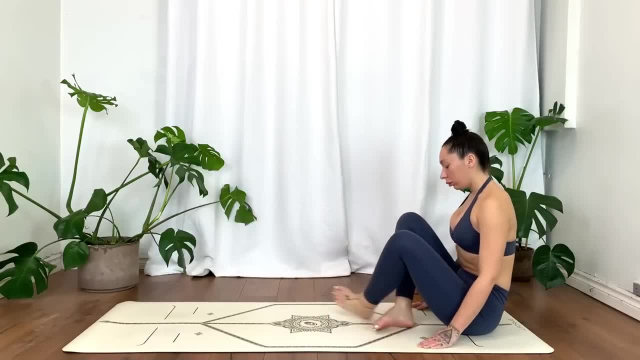 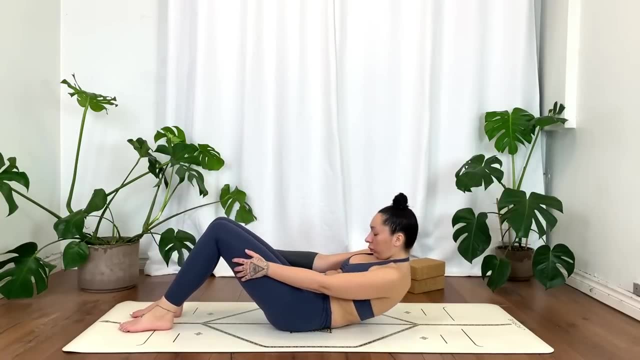 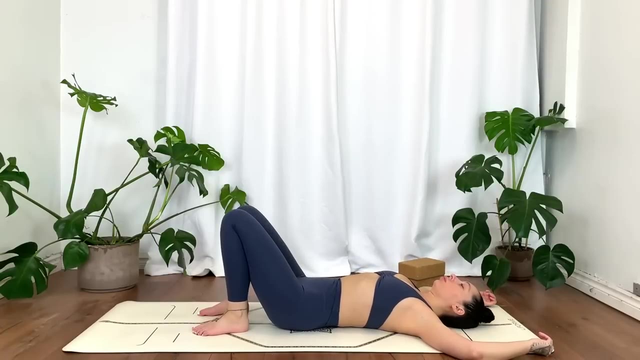 time and take your own time as you relax and relax. as you relax and relax and relax, We'll make our way down to our backs. Back stays flat on the mat as you drop both knees over towards the left for a supine twist. Option here: to place pillows between the knees and underneath that left knee for added height. 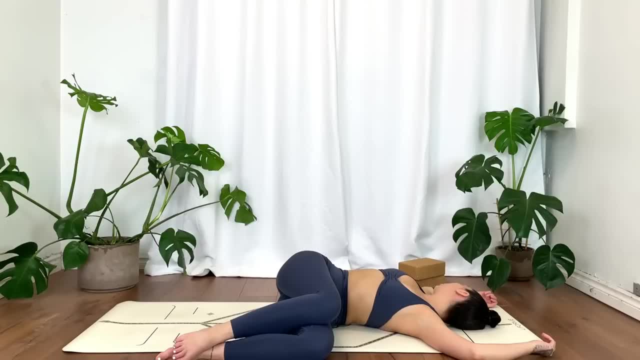 You can even place a pillow underneath the right shoulder for less of a twist. Again, working with the breath: all about the breath here. Allow it to create that space. Allow your exhales to completely let go here, softening the body wherever you can. 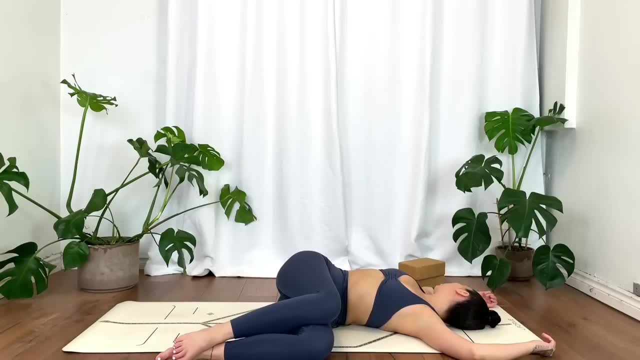 Exhaling, let it release. Exhaling- come back to that position. Exhaling: come back to that position Once again, coming back to that position All the way down. Exhaling- come back to that position. 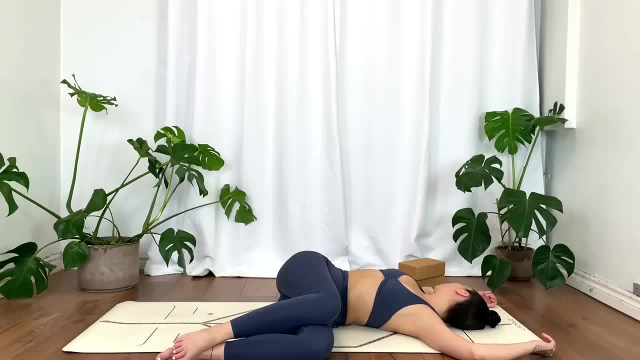 As you exhale, handle the body inside of you Exhaling. come back to that position. Last bend to yourself. Last bend and we'll lift up the knees, take it over towards the right same thing. utilize your inhales, create that space. exhale to completely let go here. 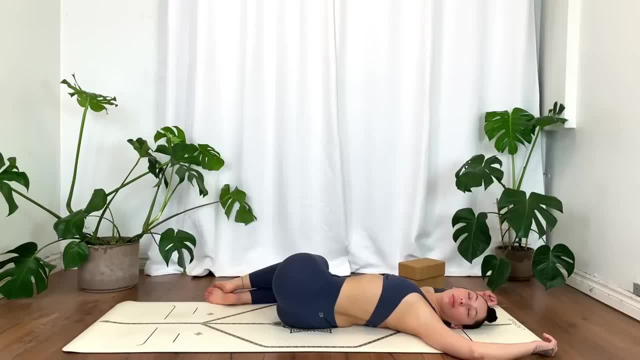 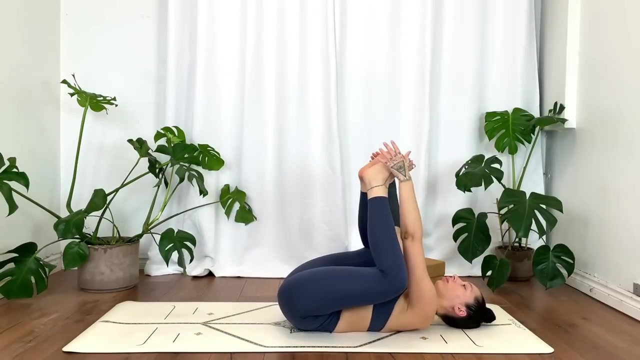 you, you and we'll gently lift the knees, hug the knees in towards the chest, grabbing the outer edges of the feet. you can keep the bottoms of feet to touch or open the feet for happy baby. you can gently rock side to side. perfect. go ahead and give your knees a hug, big squeeze, maybe even still gently. 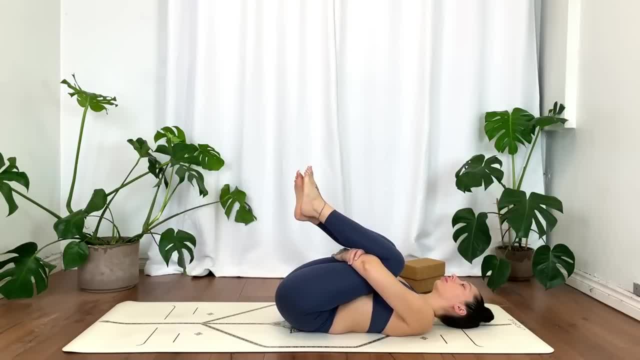 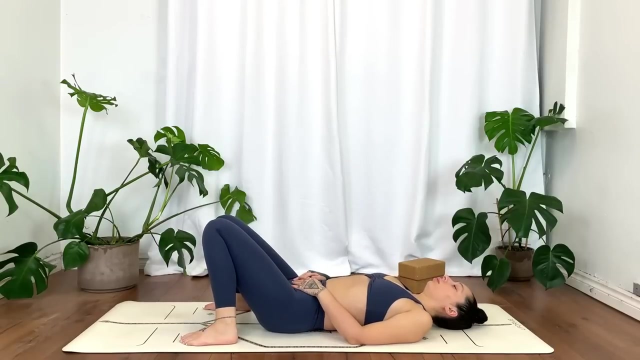 rocking side to side and then we'll plant the feet on the mat. you can let the knees kind of rest against each other, maybe placing your hands on your belly, drawing the breath into the belly. nice and tight big inhale, exhaling. once again, soften the belly. 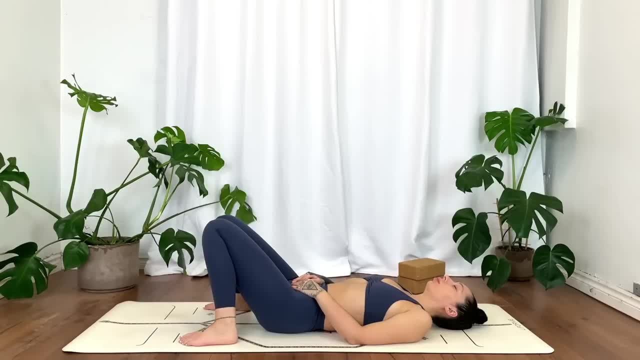 maybe you're feeling digestion happening, just observing, observing the body here. no tension in the belly, no tension in the ribs, the lower back, no tension in the hips or the knees, the thighs. no tension in the glutes, no tension in the hips or the knees, the thighs. 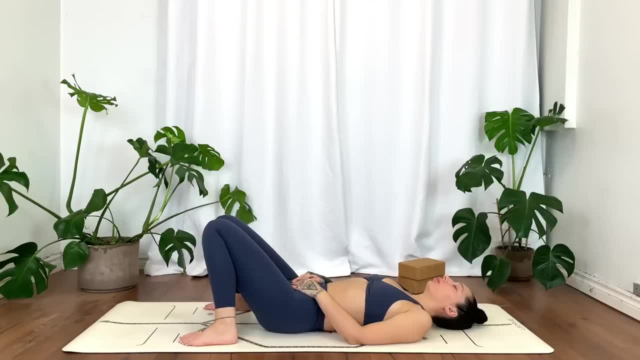 lifted back and relaxed, lifting hips to keep the breathing ingredients. your hands open, pushing back, getting really light, breathing against the thighs, our sentimental body. there's no tension and it's not even opening up our world. your energy, everything you're living, your bright, your energy, your just. 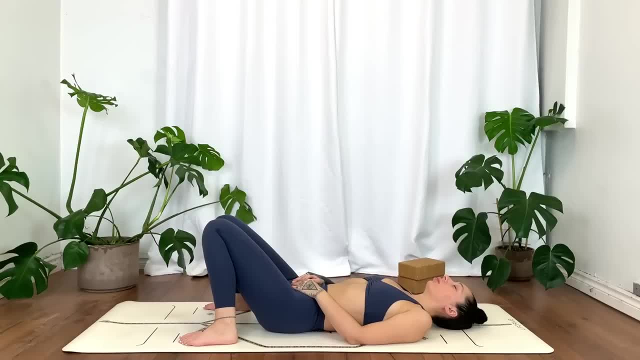 how are you doing? why are you doing this? Thank you, Thank you, Thank you. We'll gently begin to wake up the body rocking the knees side to side. Whenever you're ready, we'll roll over towards our right, full inhale. 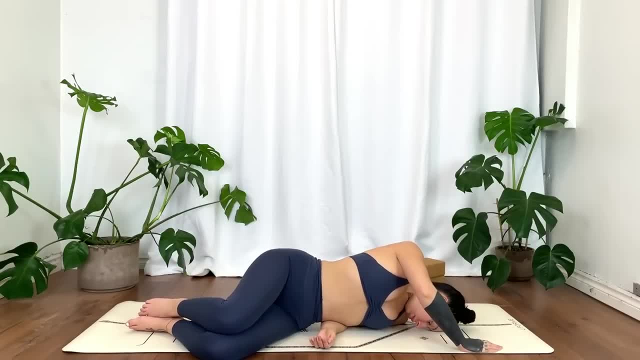 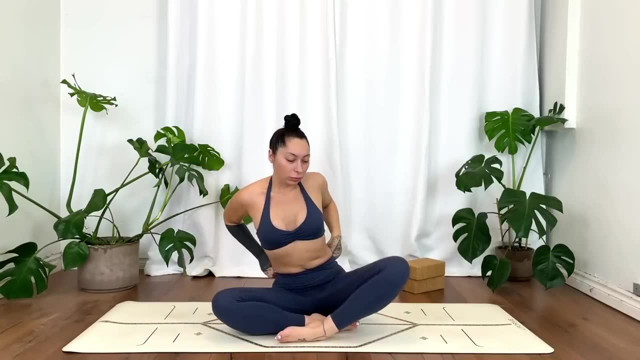 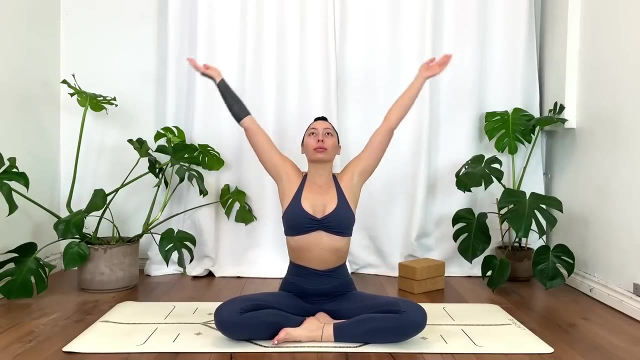 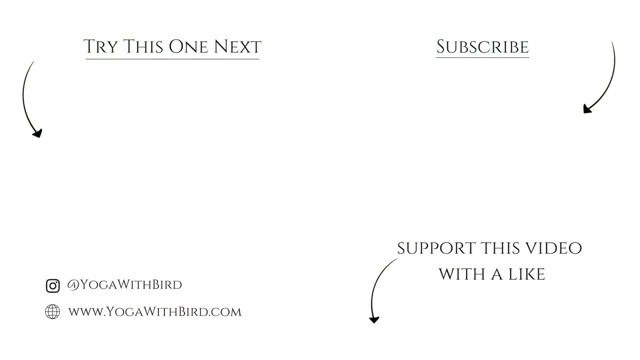 And exhale. We'll come to a comfortable seat Inhaling the hands up overhead. Exhale heart center. Thank you for joining Namaste. If you enjoyed this video, don't forget to like it below. Subscribe to my channel. 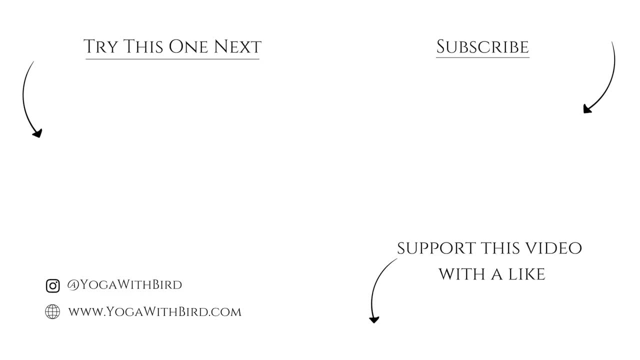 And hit the bell icon so you don't miss any updates on future videos and live streams.